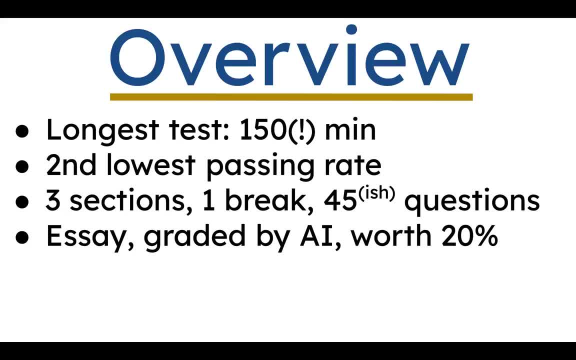 algorithm and it's worth about 20% of your total score. It usually costs 30 to 40 bucks depending on what state you live in. You can go online to see how much it costs in your state. So what does it cover? 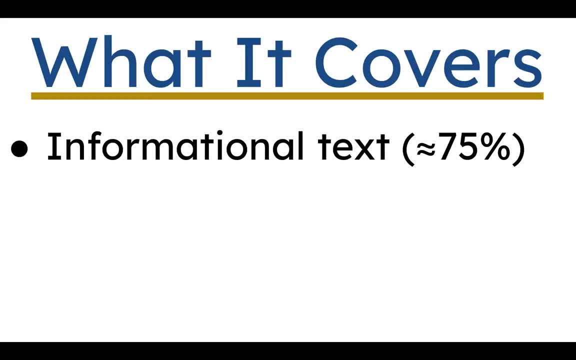 It covers mostly 75% informational texts, And informational text is like this kind of stuff: Speeches, articles, historical documents, instruction manuals, job cover letters, office memos, things that are real-life, non-fiction writing that you might encounter. 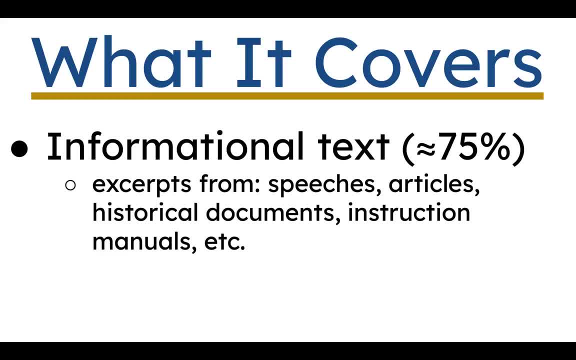 in your day-to-day life. They want you to be able to reason through how this kind of language is translated. They want you to be able to understand how it's trying to achieve its object, how it's trying to get done, whatever it's trying to do. That leaves about 25%- one-fourth for literary texts, which 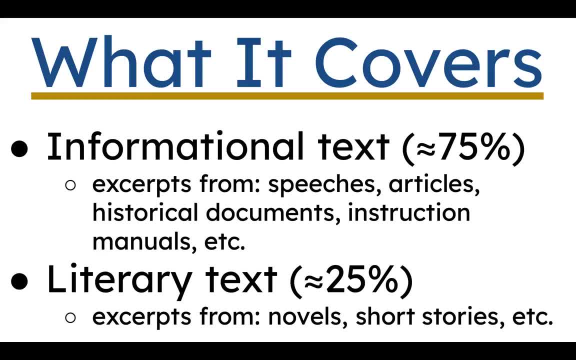 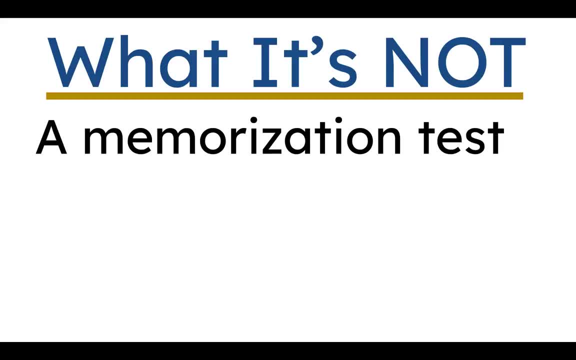 are the sort of novels and short stories that high school English classes make you read. So what is it not? It is not a memorization test. just like any of the other tests, You don't have to memorize pretty much anything. So what is it not? It is not a memorization test. just like any of the other tests, You don't have to memorize pretty much anything. So what is it not? It is not a memorization test. just like any of the other tests. You don't have to memorize pretty much anything. So what is it not? It is not a memorization test. just like any of the other tests. You don't have to memorize pretty much anything. 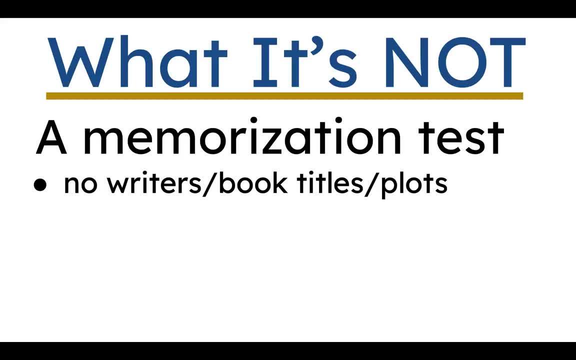 There won't be a question. you know who wrote The Tell-Tale Heart or what century was Shakespeare born in? like none of that stuff, It's also not a lit exam, so there won't be any Shakespeare or really anyone whose writing is. 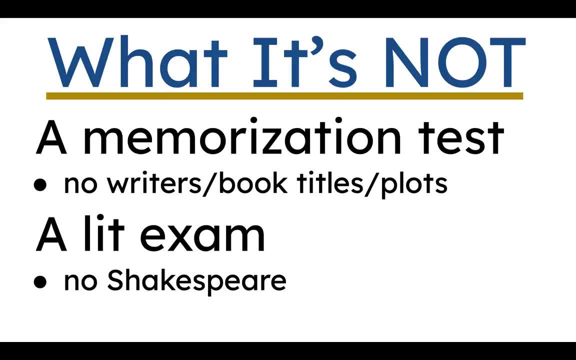 so hard that they need to have little footnotes to explain what the different words mean. Nothing like that. There's also going to be no questions about literary or poetry definitions. They won't um ask you what a metaphor is, or an analogy, or iambic pentameter, all these sort of like lit. 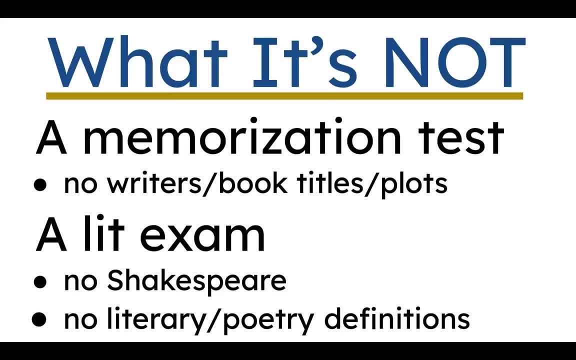 terms that maybe you would have had to study for on a high school test. They won't ask you these things. However, there's a little asterisk ding. should have made a sound effect when that appeared, but um, it doesn't hurt to know these things If you know figurative language and what. 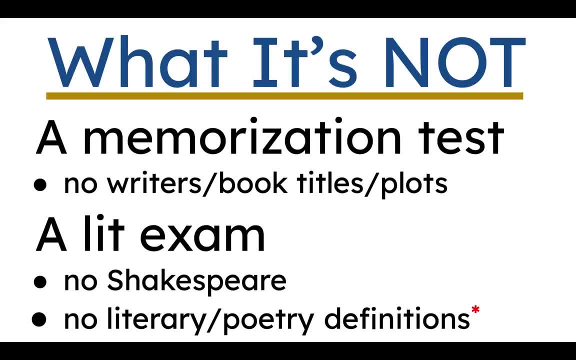 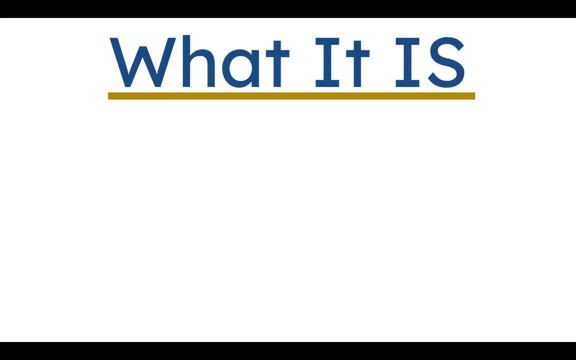 figurative language is, and some of the terms that um apply to that analogy, metaphor, simile, that that can help you, That's, that's not unhelpful, All right. um, also what this test is. 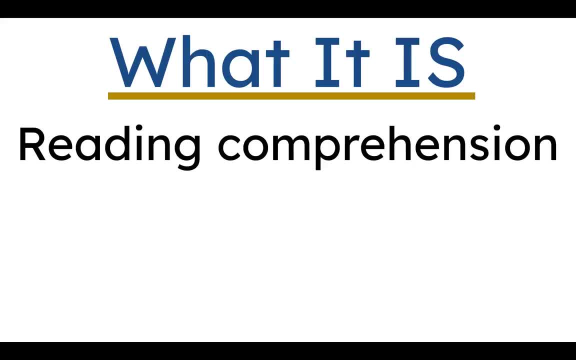 uh, it is a reading comprehension test. uh, just like the other three. Science test is a reading comprehension test about science. The social studies is a reading comprehension test about government and history and economics and geography. This is a reading comprehension test about. 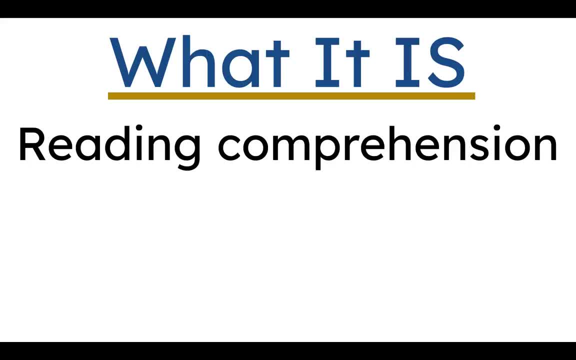 pretty much any other kind of writing that you would encounter, and you might even encounter some social studies-ish stuff or even some science-ish stuff- The sort of things that you'll be asked to do. you'll be given a chunk of text. 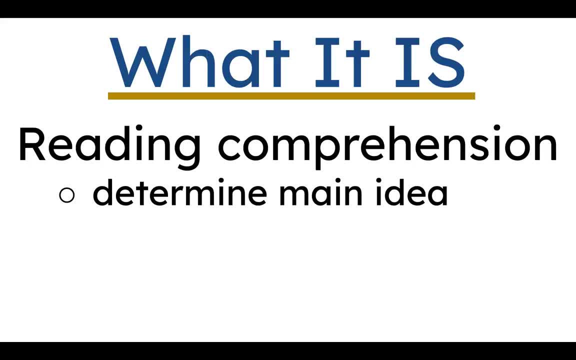 and probably the most common and most fundamental question they'll ask you is: what is the main idea of this text? What is the thing that the author wants you to know? um, after reading this, They might also ask you to understand or identify what the purpose of what you just wrote was. Is it? 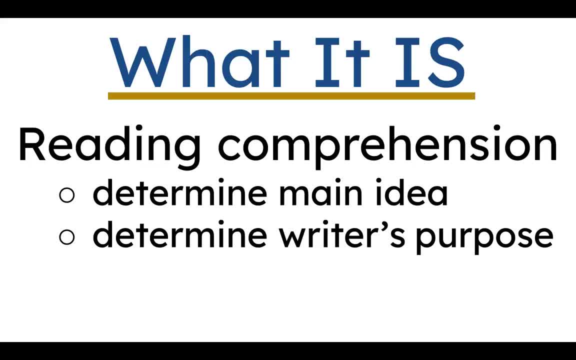 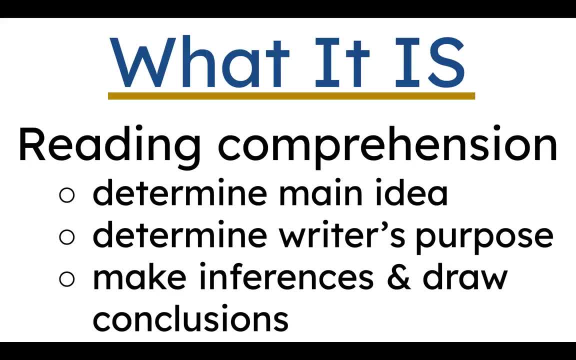 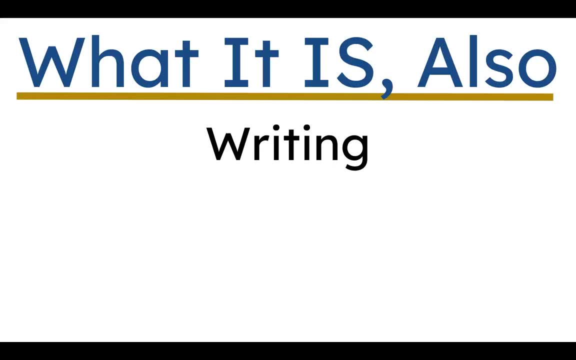 There'll be. the author will be talking about something, but not come right out and say it. It'll be up to you to make an inference and draw a conclusion about what the author's really talking about. It is also also also a writing test. This is the only test that has writing in it. 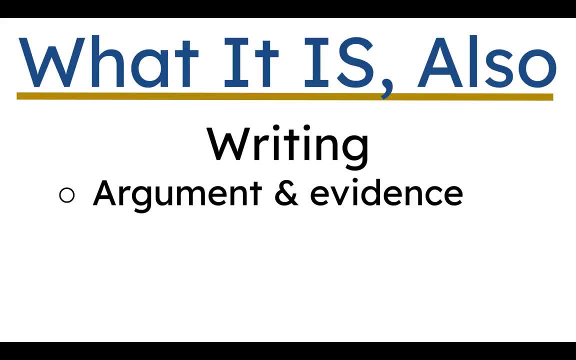 And there are three categories that your writing will be judged on. The first one is argument and evidence. Can you make a clear, coherent argument about something and then back it up with quotes from the text and examples from the text? Can you organize your writing well? Can you um start with an introduction that has a thesis in it? 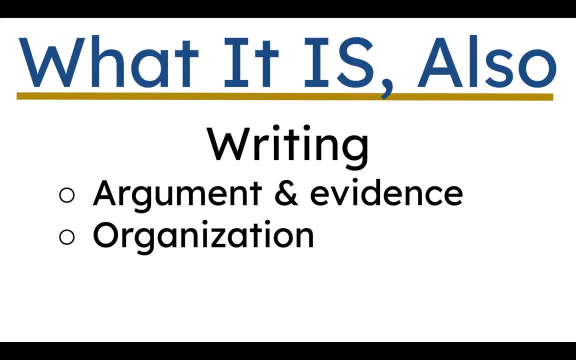 have a couple of body paragraphs that expand on the thesis and then wrap it all together. wrap it up all together with a conclusion. And finally, how good are you with language Um? are you confident? Do you mix up your um syntax? Do you use fancy vocabulary words? 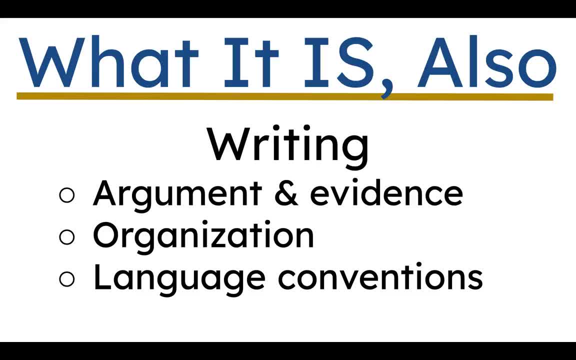 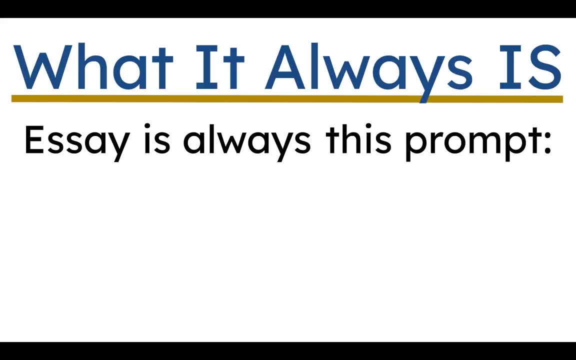 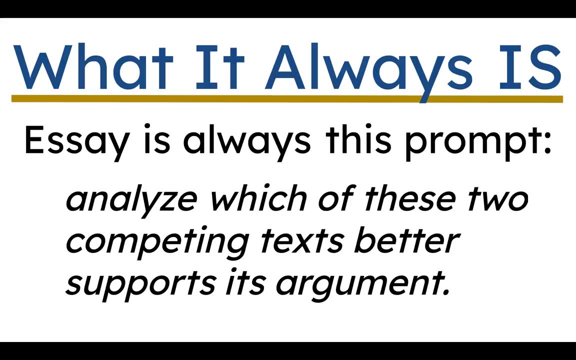 Or does your writing look like a text message or a tweet? The good thing about the writing for us is that the essay is always the same. The prompt is always this: Analyze which of these two competing texts better supports its argument. 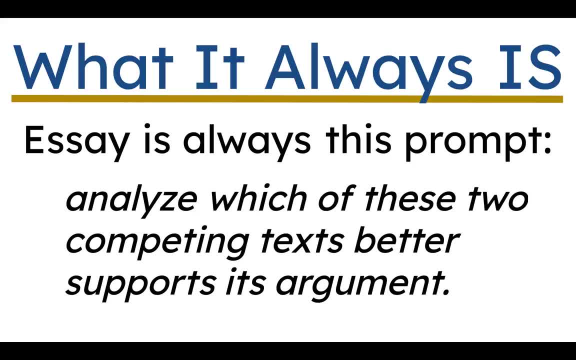 So they're going to give you a pro and a con, usually about something. One guy will say: I think summer is the most wonderful month, the most wonderful season of the year, And someone else will write an op-ed opinion piece that says: I think winter is the. 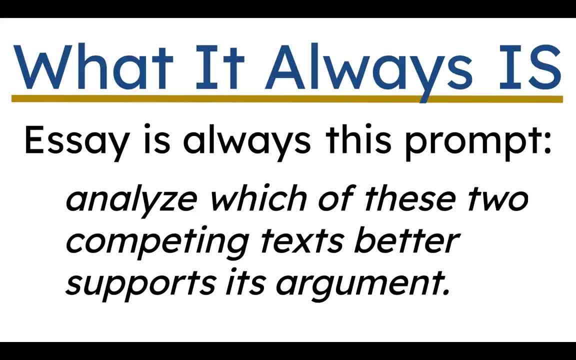 best season, And then it will be up to you not to agree with one or the other. That will get you nowhere. It's not about your opinion. It's about which of the two people making the argument better job. which one supported his or her argument better. It won't be something as stupid. 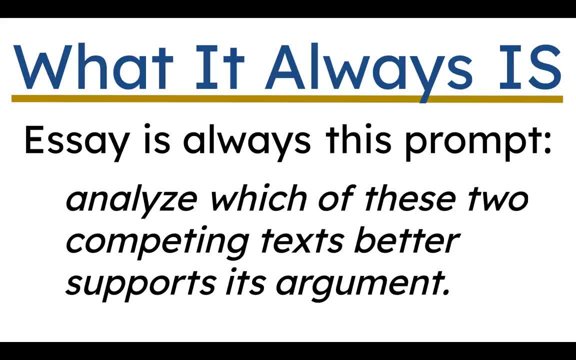 as which is the best season, but it could be the one they have on their website. the GED is something about recyclable plastic bags. Do we, should we outlaw them at supermarkets or not? Something like that And you'll be tempted to like: agree with a position because everyone. 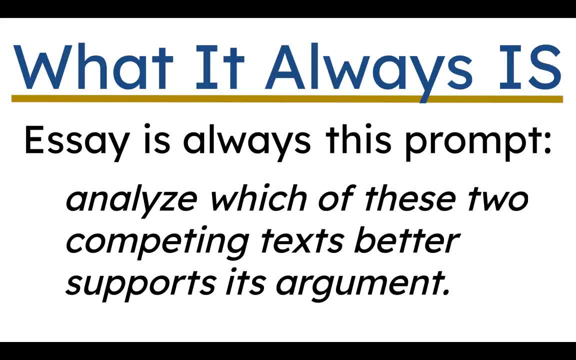 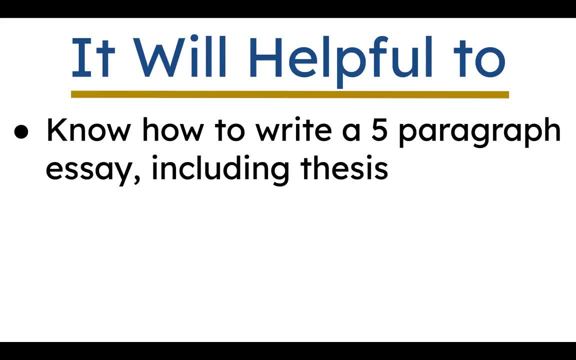 has opinions about a lot of stuff. but don't do that. All right, Some things that will be helpful to be able to do on this test. First, know how to write a five-paragraph essay including a thesis, what we were just talking about with the introduction, the body paragraphs. 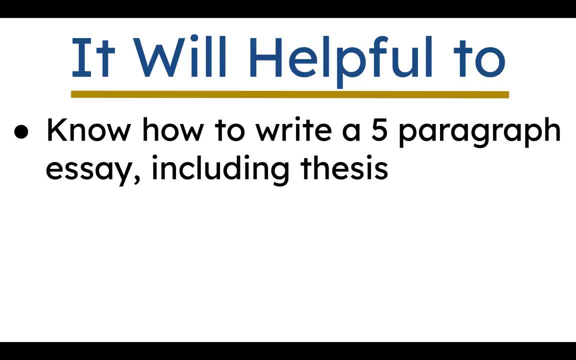 and the conclusion. There are a lot of websites and YouTube videos. I have one on my channel about this specific essay. If you know how to do it and you practice it, that's all they're looking for is a five-paragraph persuasive essay. 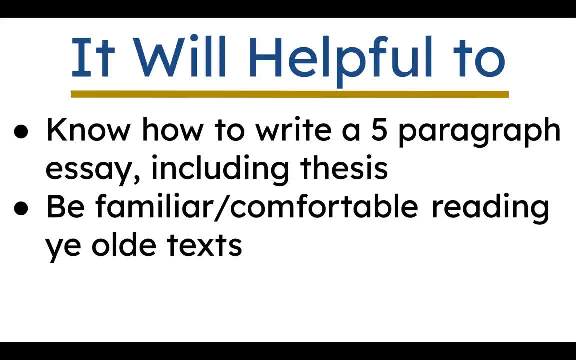 And you'll be ready for the, for the writing part of the test. Um, um, um. you should also maybe, if you can, practice with old stuff, olden days texts, So they might throw like the US Constitution at you. 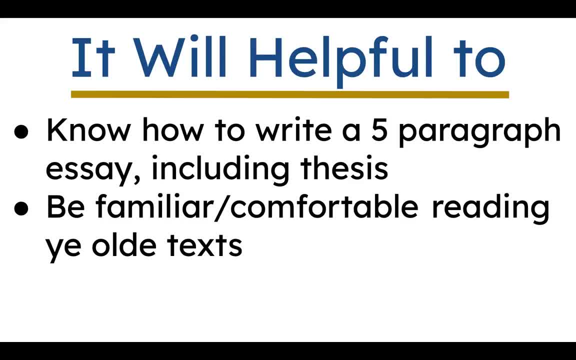 Things with like the kind of language we don't use anymore, And if you're comfortable reading something from Edgar Allan Poe, who is died in the 1800s and is pretty dense and pretty tough and uses a lot of difficult vocabulary, if you practice with that, that will help you. 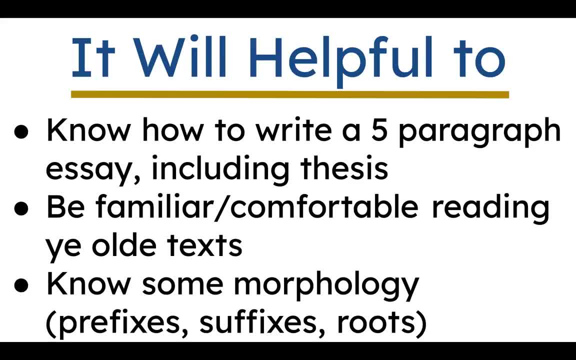 for the harder stuff that shows up on the text. um, um, Let's keep going. Um, Okay, So I'm I'm not gonna like this. I'm not gonna like this. Okay, um, okay, So I'm gonna use this. 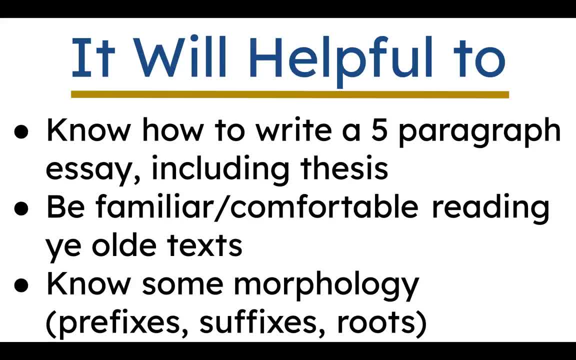 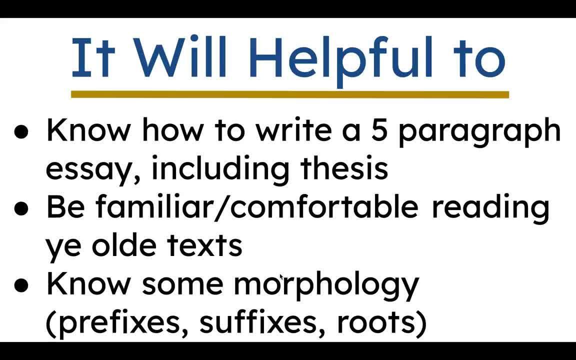 question it this summer. Um, I have two books where I suddenly wonder if I know- because I didn't show, Draw my brain a little bit- Grade, that's like beyond a shape, It's a shape that transforms into something else, metamorphosizes. So, if you can like, look at these words and kind of see where. 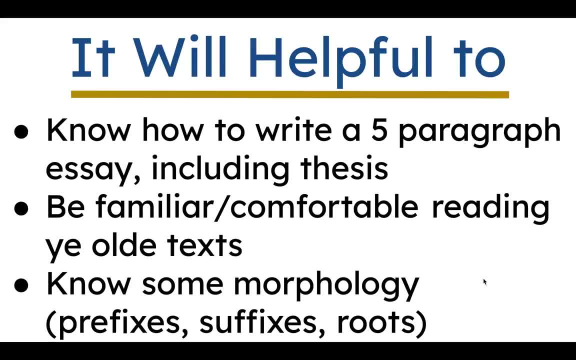 they come from. when they hit you with some difficult vocabulary, you might be able to reason your way out of it. That might be helpful. None of these things are essential. You can absolutely pass the test. having no idea how to write a five-paragraph essay, or having read nothing before 1987, or knowing no. 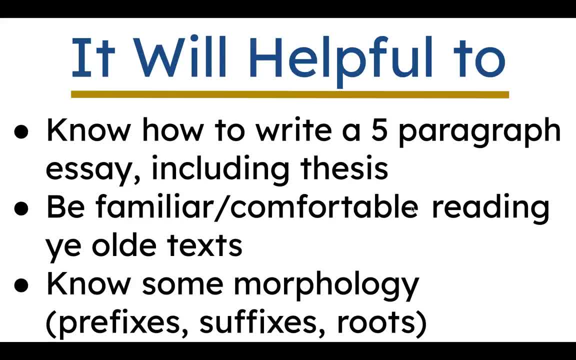 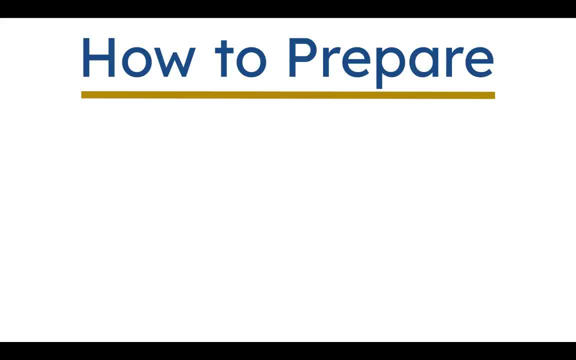 prefixes, Prefixes. The word prefix Pre means before There's another prefix in the word prefix. Alright, how do you prepare for this? It's the same for all these videos, for all four tests. You should first of all take the. 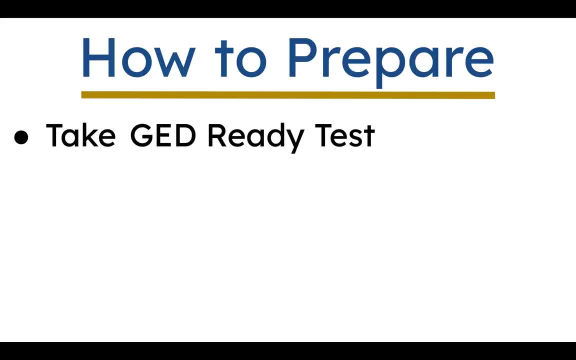 GED Re gravitational positive friends test. That will tell you how you're doing, how close you are to passing right now. It will tell you what you can work on, what skills you can study to improve that score, to get it up to passing. You can take classes, Go to. 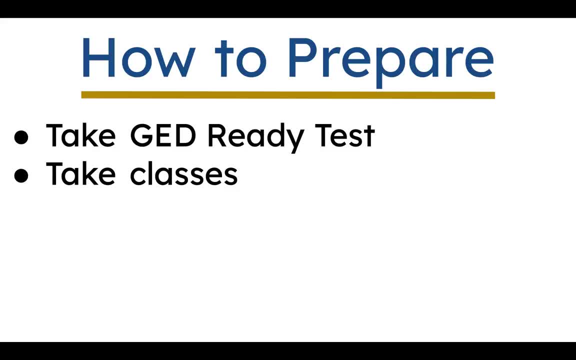 The GED Re Success button below website. enter your zip code. There may be free classes near you, or there are classes you could pay for online or classes you might be able to pay for at a community college near you- Lots of. 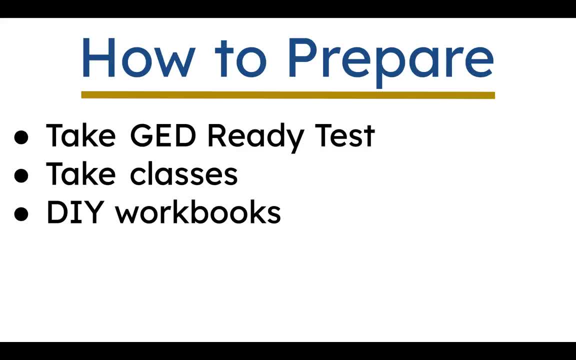 different stuff. You can get a book from Target or Walmart or Amazon- the Kaplan book or the Stackbond workbooks- All of those are good. if you're a self-motivated kind of person- You have made it this far on the YouTube video, so good for you. You obviously can watch some. 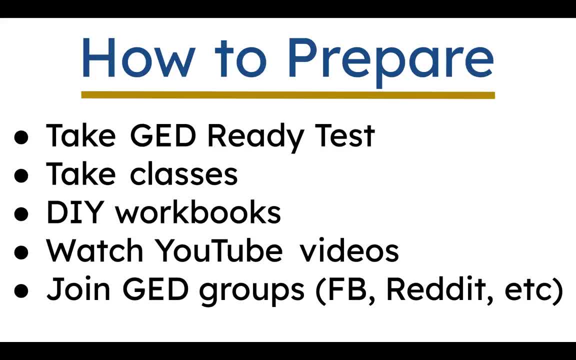 YouTube videos. You can also join GED groups on Facebook or Reddit if you want. like a positive, mutually supporting atmosphere where people kind of encourage each other to keep going with this stuff. All right, that is an overview of the test- how to prepare for it. Let's look at a typical 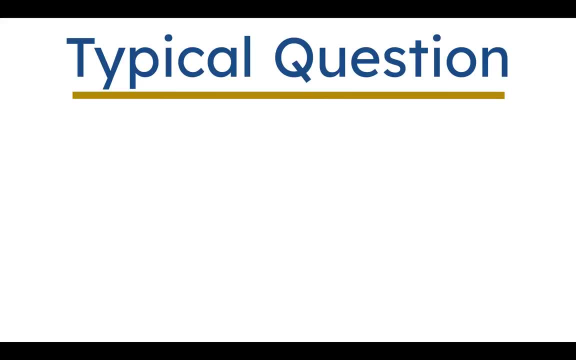 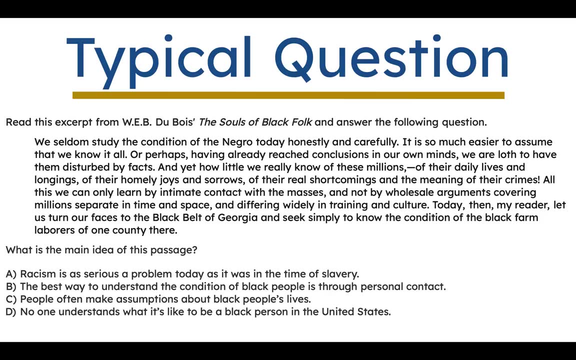 question. I'm not going to read through this. I would totally heartily encourage you to pause the video here. Read this question over and see if you can get an answer, and I'll go through it and talk about how I would approach this. Okay, unpaused, The first thing I'm going to do is read the question. 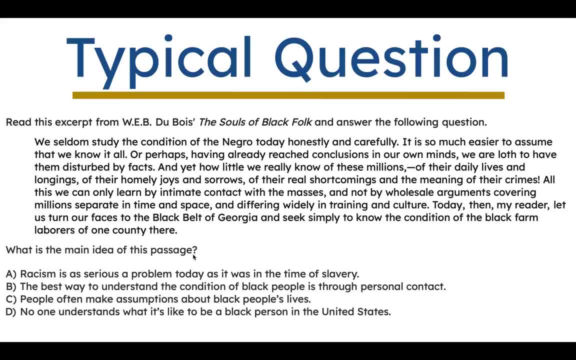 and the question really is this: What is the main idea of the passage? So sometimes it helps when you read a question before you read the big chunk of text in the middle. It will help you know what you're looking for when you start. 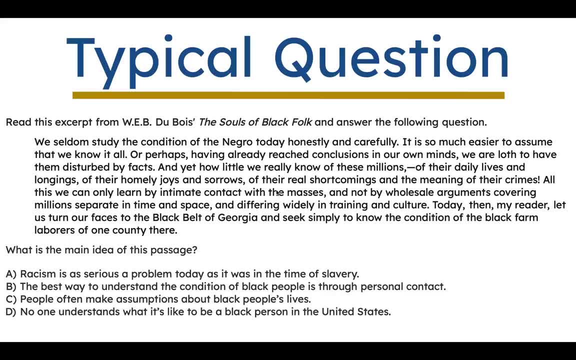 Reading This one is pretty general. What's the main idea? What does the author want me, the reader, to come away from this paragraph understanding? And I'm going to look not for the right answer, I'm going to look for the wrong answer so I can eliminate some of these possibilities and improve. 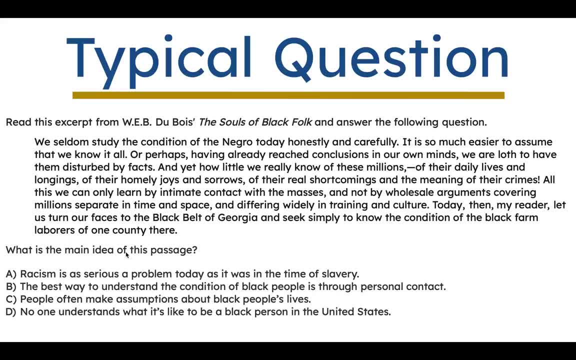 my chances of getting it right through process of elimination. So the first one says racism is as serious a problem today as it was in the time of slavery. So nothing specifically jumped out at me in this paragraph about racism. I don't really see that. 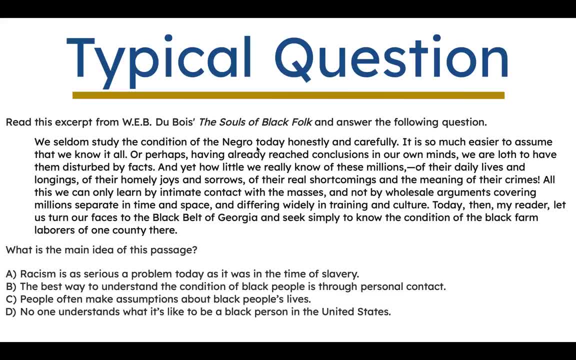 this is necessarily about racism. It does use the word negro, and negro is a word that is not offensive today, but definitely dated. It's a word we nobody- nobody, it seems even to say. it seems super weird, But that's a different word than the offensive one, So it's not. 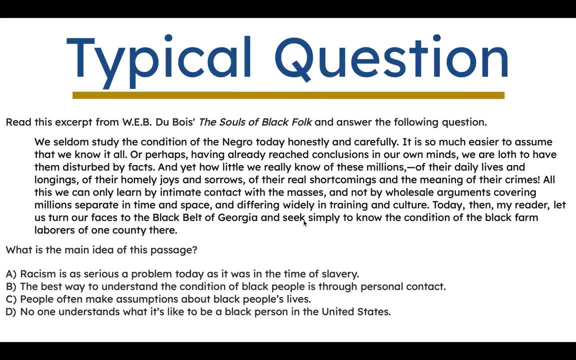 necessarily a word that is offensive today, but definitely dated. It's a word that is not offensive today, but definitely dated. It's a word that is not offensive today, but definitely dated. And it's also about slavery. I don't really see much about slavery in here either, And if I'm going to read: 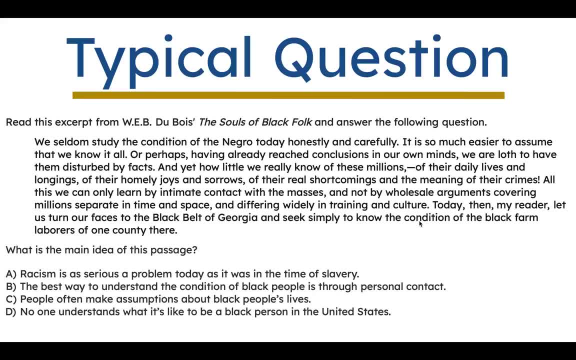 the end here there's an inference I can make that will tell me it's not about slavery. This is sort of in the make inferences category of questions. It says here: let us turn our faces to the black belt of Georgia and seek simply to know the condition of the black farm laborers of one. 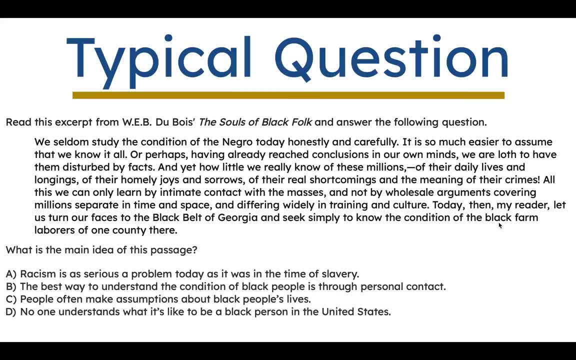 county there. Well, if this were during the time of slavery, they wouldn't be referred to in Georgia as laborers, They would be slaves. So this is after slavery ended. So there's too many- excuse me- red flags about racism and slavery. I'm not. 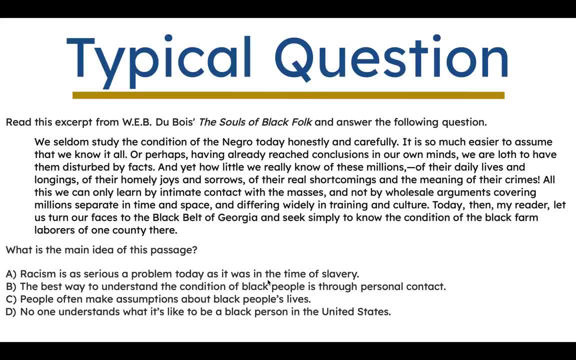 I'm going to eliminate it. It's not A. The best way to understand the condition of black people is through personal contact. That one. if you look in the middle of the paragraph, it says all this: we can only learn by intimate contact. 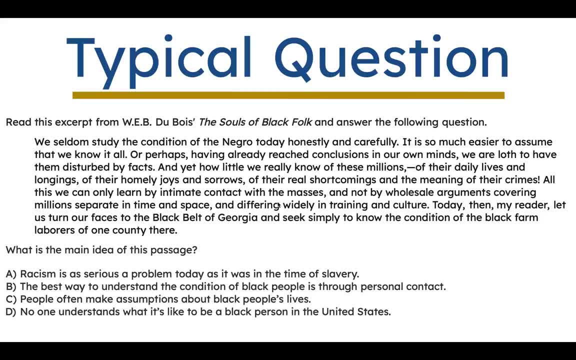 with the masses and not by wholesale arguments covering millions separate in time and space, So that one seems okay. Is that the main idea? I don't know. It's definitely being talked about, unlike slavery and racism, So I'm going to keep that one around. B to the next round. 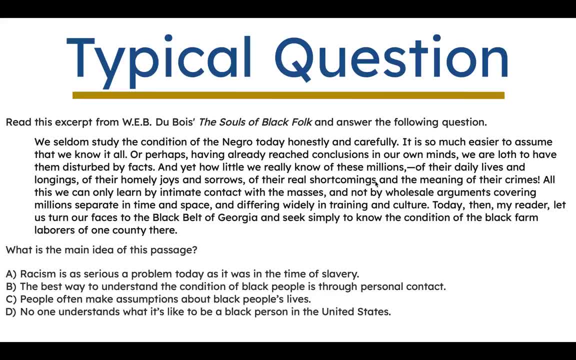 C, people often make assumptions about black people's lives. Well, it does say it is so much easier to assume that we know all about the condition of black folks, or perhaps, having already reached conclusions in our mind, we are loathe to have them disturbed by facts. That's about making assumptions, Is that? 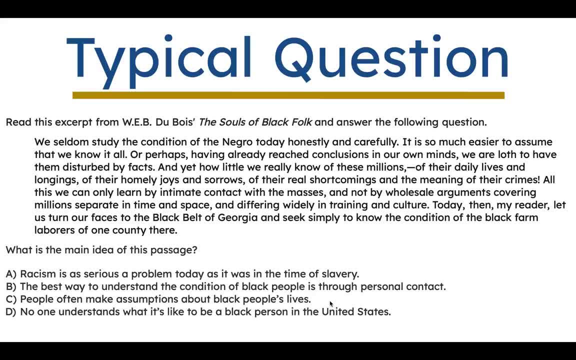 the main idea. I don't know, But also like B is a pretty solid answer. So B and C, I'm going to keep around D. no one understand what it's like to be a black person in the United States, So 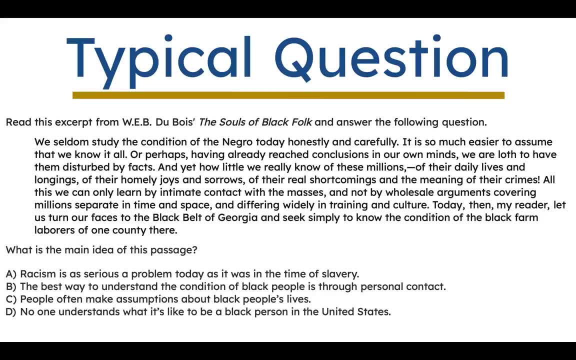 again. there's some red flags here with D, And the first is this: no one understands. Whenever I see an answer that is no one or everyone, or never or always, it's one of those like all or nothing, black and white answers. I really look very carefully to make sure. 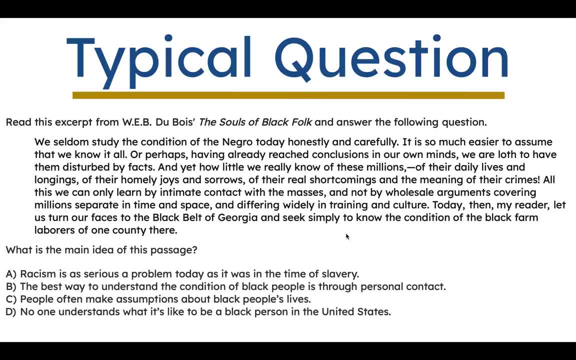 it really is all or nothing. No one understands what it's like to be a black person in the United States. There's a lot of black people in the United States who probably have a pretty good idea of what it's like to be a black person in the United States, And you may or may not know. 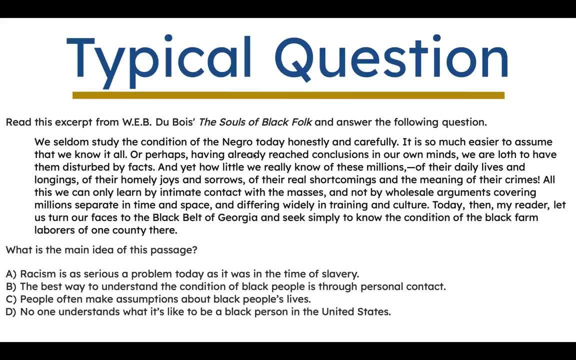 this, but WEB Du Bois is himself a black man, So that one. just it smells wrong. You know, it's not going to be, it's not going to be D, So it's either B or C. Which of these two?